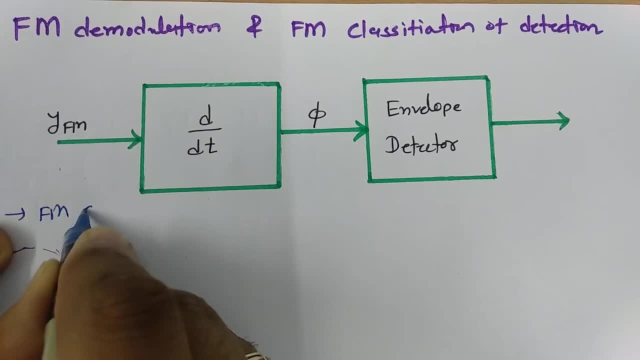 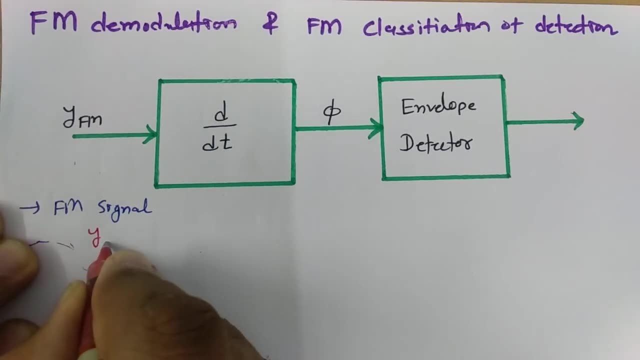 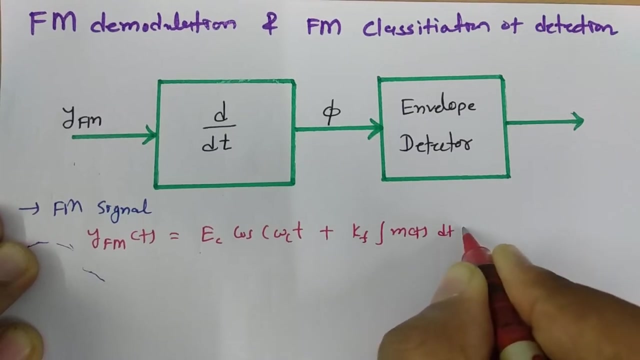 where FM signal, so that we have already seen that FM signal is. if I say it is Y of FM, of T, then that is E, E, C, cos of Omega, C, T, plus K, F into integration: M, T, D, T. This is our basic FM signal. Now 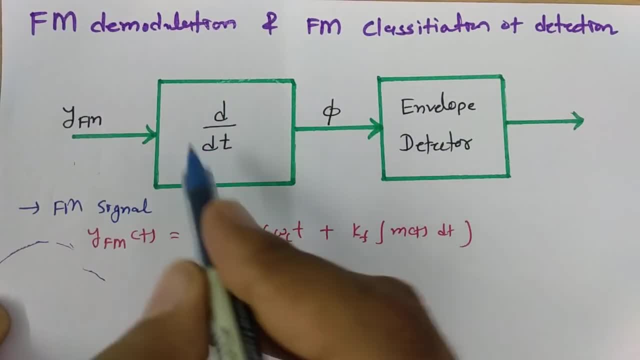 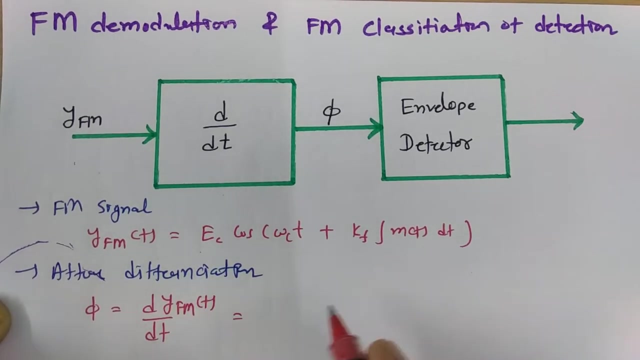 as I have told, we just give this signal to differentiator. So after differentiation we'll be finding that signal is Phi And that is D by D, T of Y, of FM, of T. So if we do this differentiation, then this E C will be constant. Just take it outside. 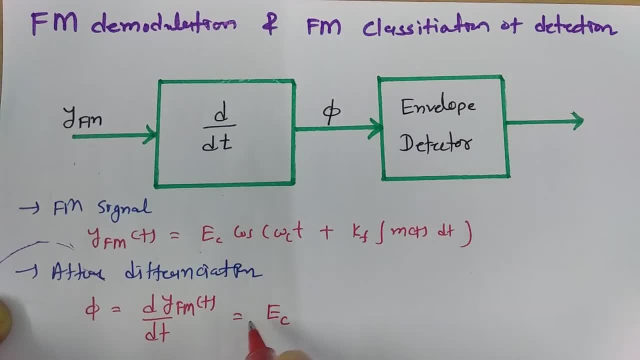 and this cos that will be minus sign. So I'm just placing minus sign over here and this angle that again will be getting differentiated with respect to time. So that will be Omega C- T, Whereas T is having one differentiation. so Omega C plus K, F, integration, M, T, D, T It's. 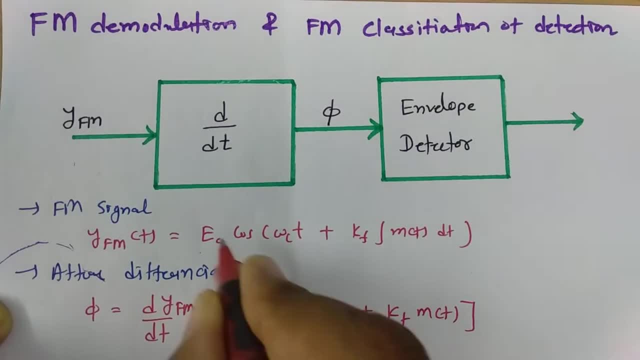 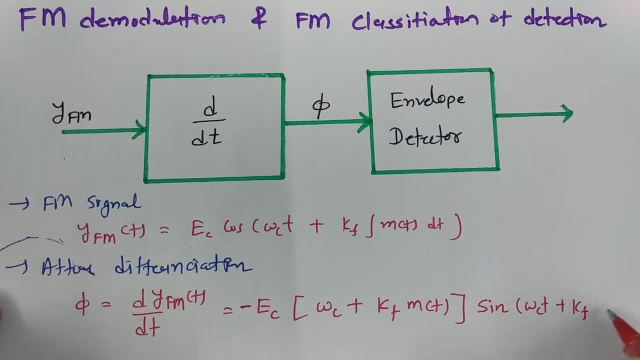 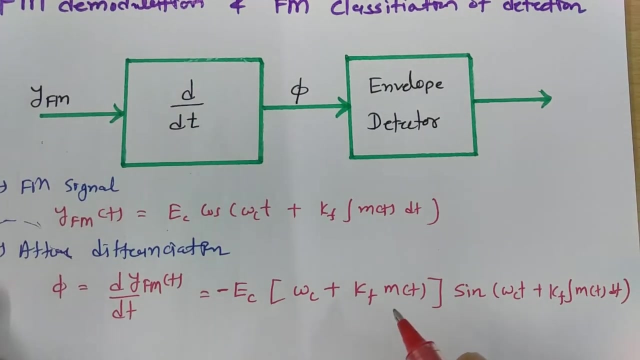 differentiation will be M, T and this cos is sign Omega C, T plus K, F, integration M, T, D, T. So this is what the basic signal that we have after differentiation. Now, if we take, Now, if you see this signal, then this signal is having similar understanding as we have. 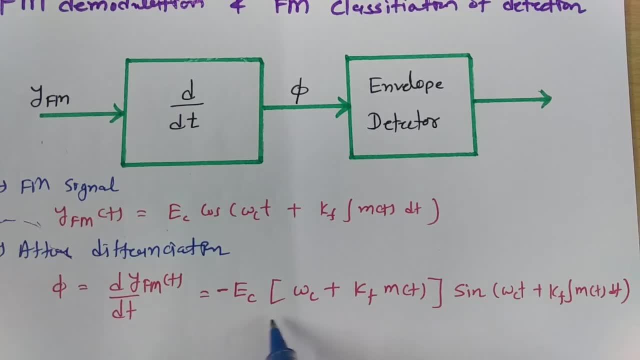 seen it in AM signal. So this is what one can see. it is similar to AM signal And this is what envelope, which is what one can say. So this is even envelope. Now, over here we are delivered to detect this envelope. So if we have envelope detector, then after then, so we can be able to extract this information. 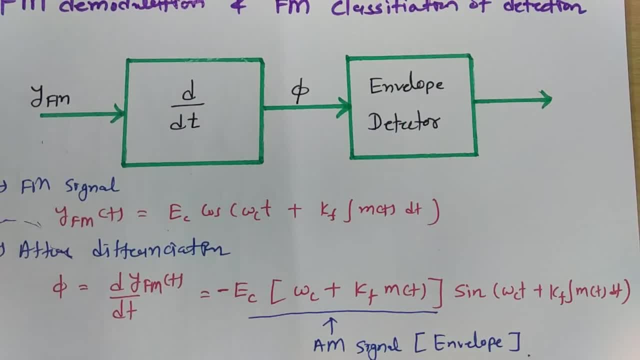 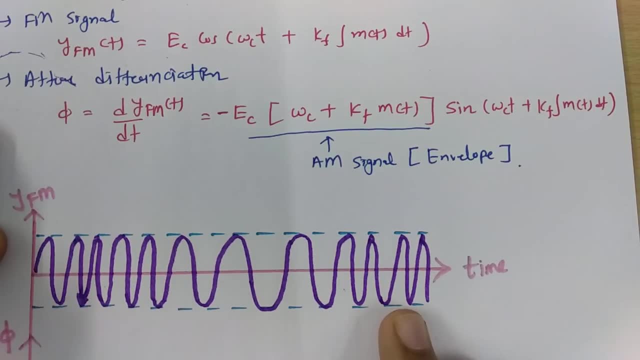 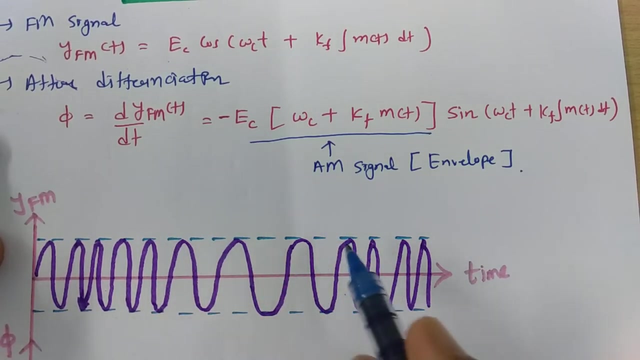 because of envelope detector. Now see before I explain how things are happening inside. let us try to understand. what is that FM signal? So if you see its waveform, Then waveform will be like this: where over here frequency is high and over here frequency is low. 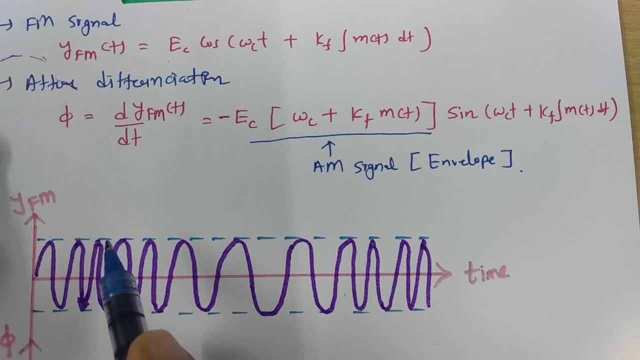 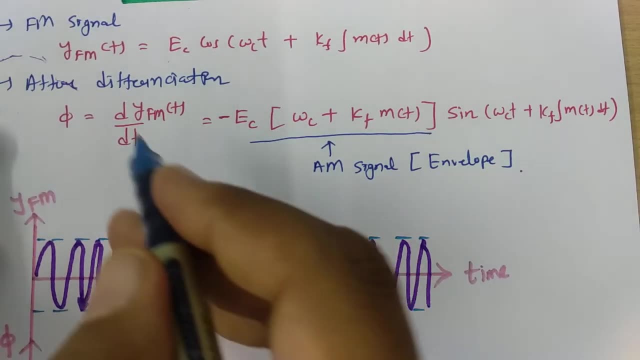 And, as you can see my previous session I have already explained: if frequency is high, it means there is higher amplitude, and if frequency is low, it means there is lower amplitude. So when you differentiate this signal with respect to time, it signal will be like this: 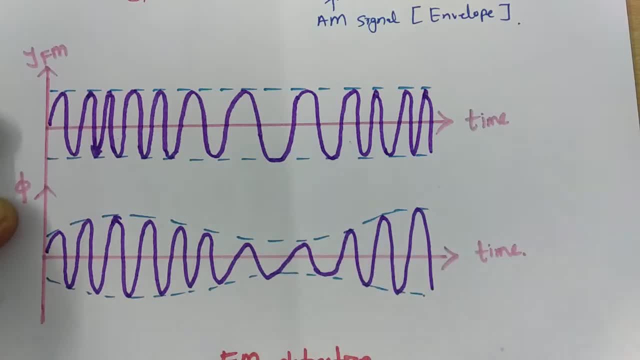 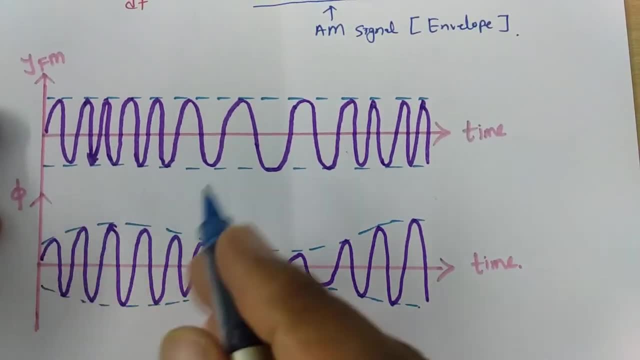 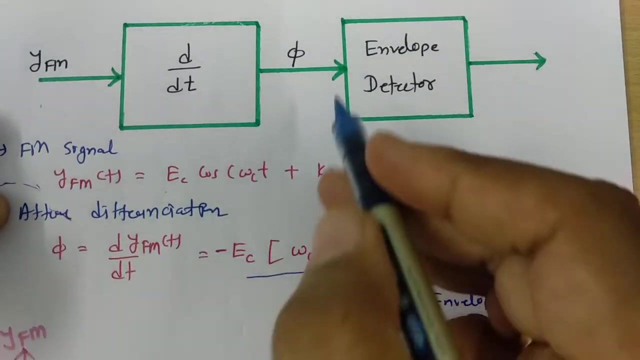 where one can see, now, amplitude is varying with respect to time. even so, that is what generation of envelope, And that envelope is this. So this is what PHY signal, that is what after differentiation of this signal. So this signal will looks like this: Now, once you pass this signal to envelope detector, we will be able to detect this envelope. 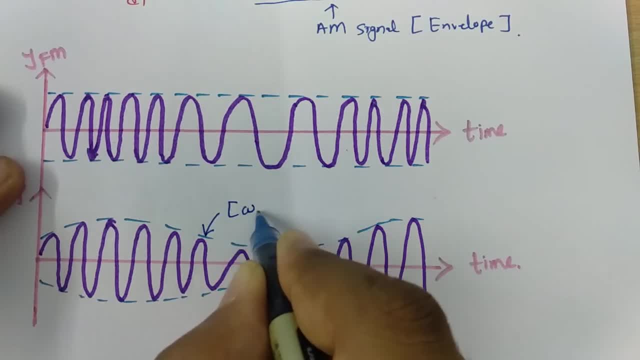 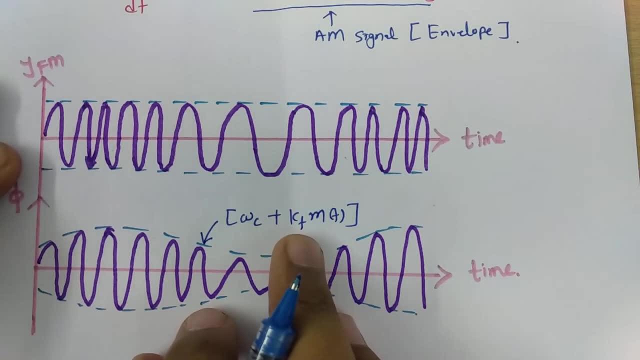 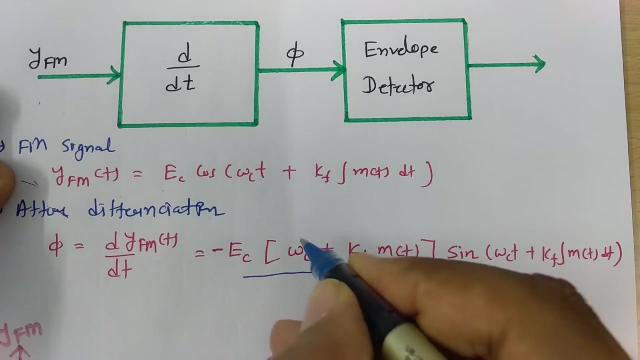 and this envelope that is omega c plus kf, into mt. Now, how to detect this envelope? So for that we have envelope detector. So for that we have envelope detector. And the basic condition for envelope detector is this omega c, this omega c that should be. 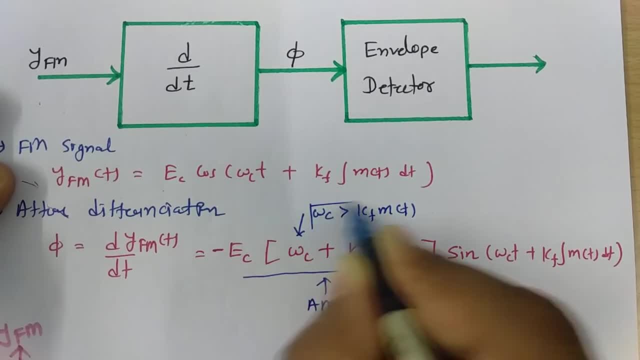 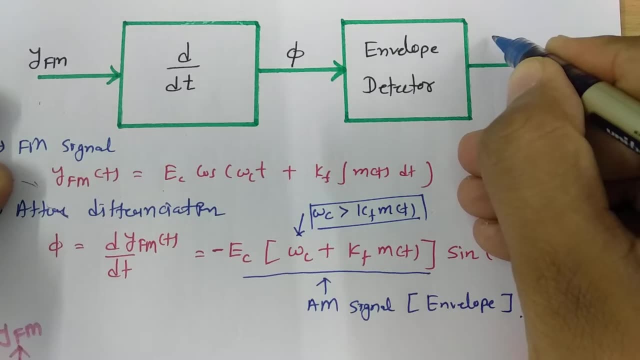 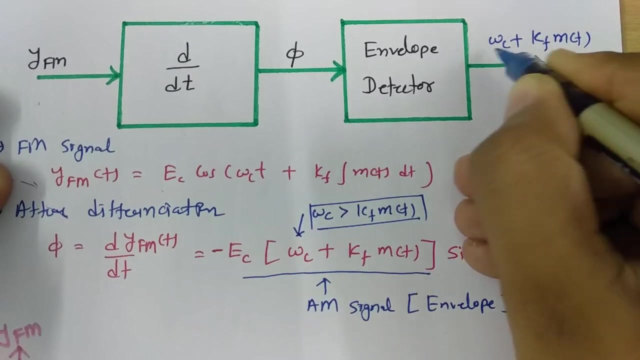 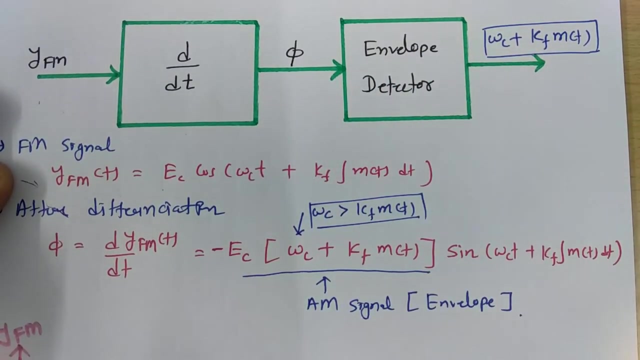 greater than kf mt. So if this condition is getting satisfied, we can easily detect this envelope by envelope detector. So over here we will be finding envelope that is omega c plus kf mt. So this will be our output And after passing this signal through envelope detector, 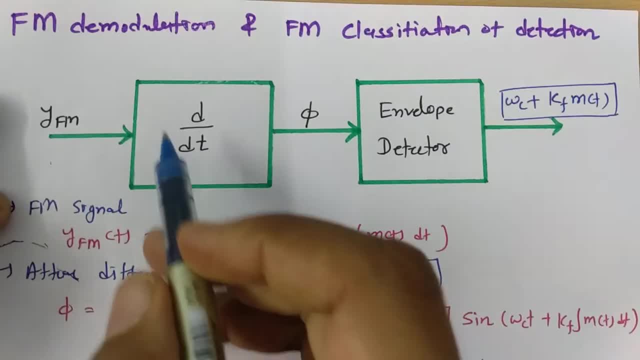 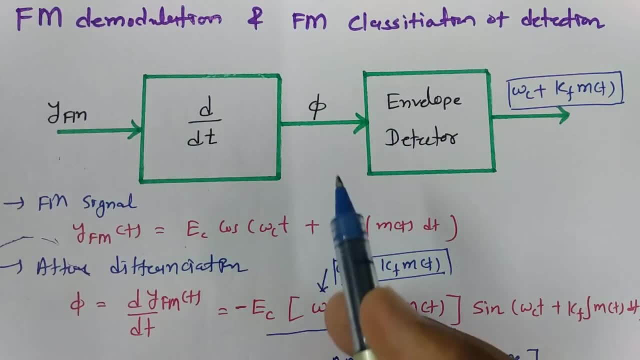 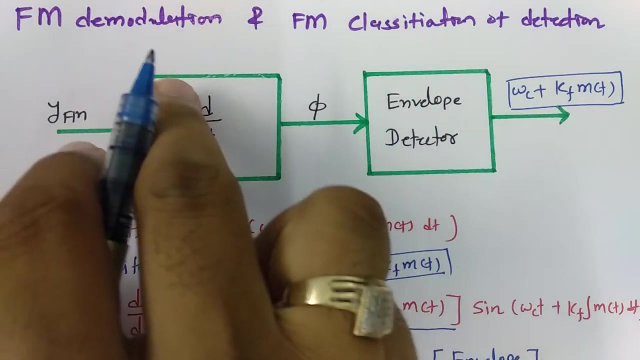 So here, basically two things that we are doing for FM demodulation. One is differentiation of FM signal, Then after we just pass it through envelope detector. So this process that we need to understand when we classified FM detection And this is what we are utilizing in different methods. 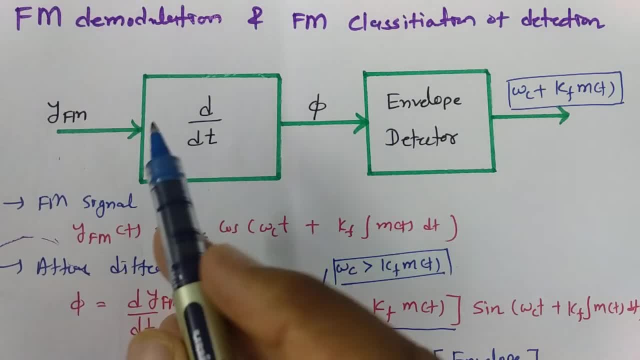 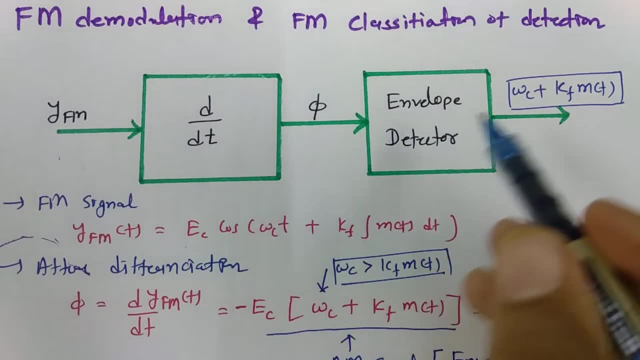 So one should have basic understanding like see how we detect FM signal. So FM signal, This signal is getting differentiated first And then we just pass it through envelope detector And this is what our signal after envelope detector. After this one can use high pass filter or capacitor to extract mt.